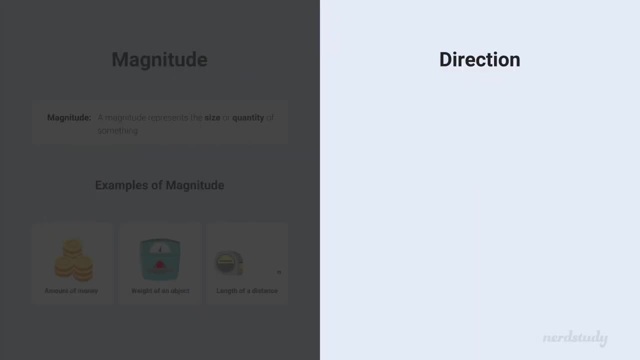 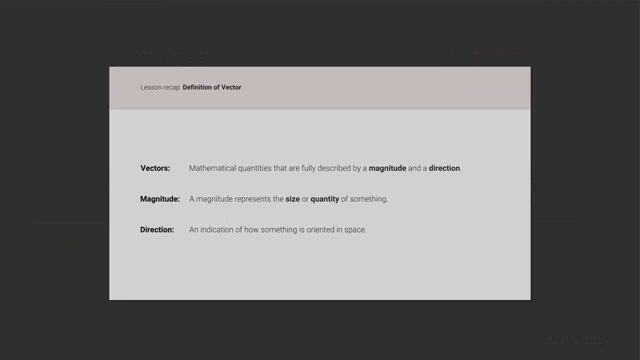 And what about direction? Well, that's simple. It's an indication of how something is oriented in space. Examples are right and left, up and down, or even east and west, as well as north and south. In mathematics, variables that are vectors usually have an arrow on top of them. 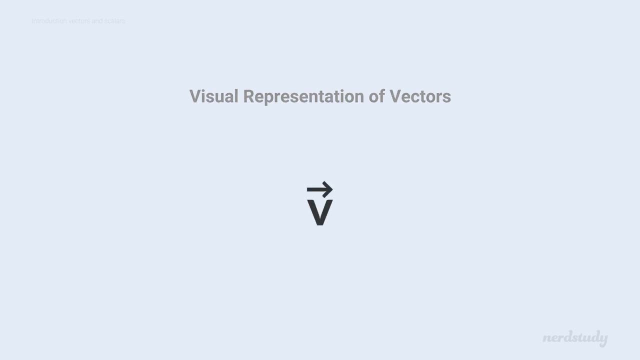 So if the variable v were a vector, we'd put an arrow above it like this, to represent that it is a vector, And that's in fact a vector quantity- Great. So here's a simple example of a vector. 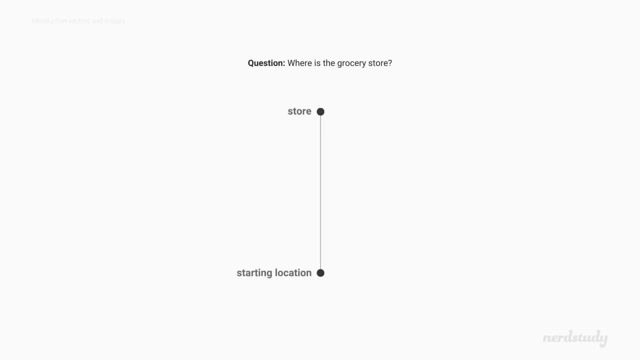 Suppose a friend is asking how to get to the grocery store and we tell them it's half a kilometer north of here. At a glance it might look like we just gave them one piece of information telling them where to go. 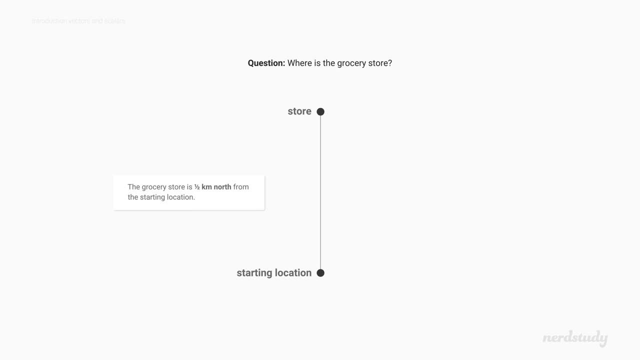 But in reality it actually consists of two pieces of information. First, we told them it's half a kilometer north of here. First, we told them it's half a kilometer north of here. Second, we also mentioned that it's north of here. 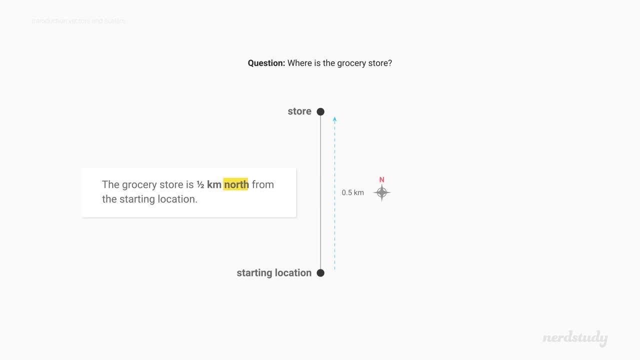 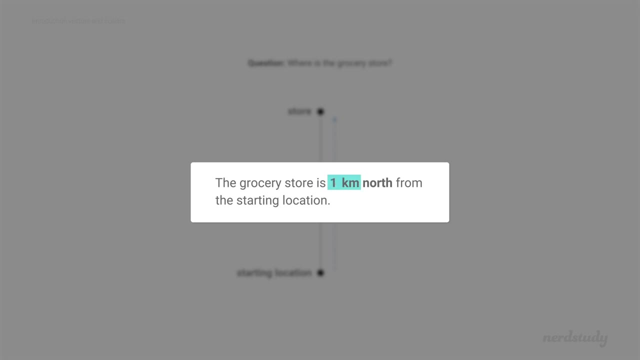 Second, we also mentioned that it's north of here. The first piece of information was the distance. It can be bigger or smaller. It's a quantity, In other words a magnitude. The second piece was obviously the direction. The second piece was obviously the direction. 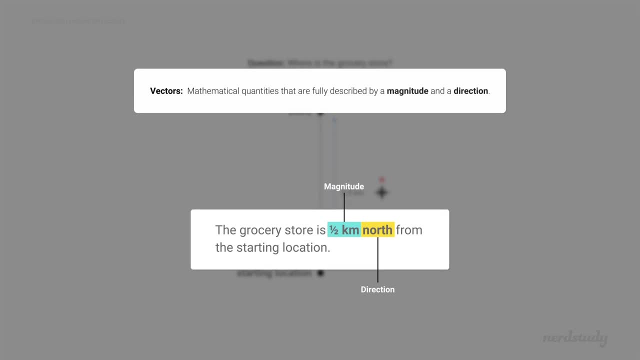 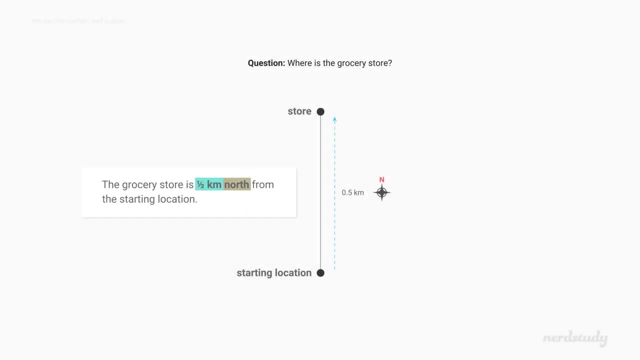 And hey, remember what a vector is, Something that has magnitude and direction, Something that has magnitude and direction. So when we said it's half a kilometer north of here, we were really giving our friend the vector 0.5 kilometers north. 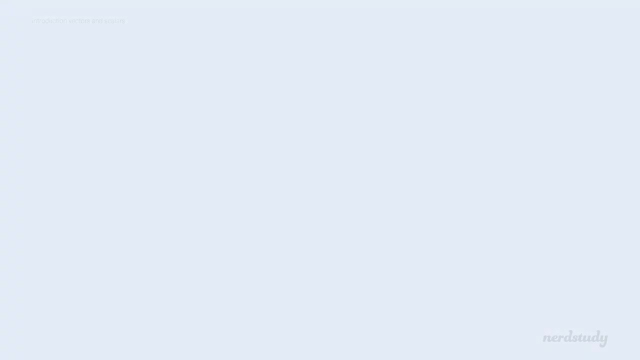 Awesome. Alright. now say, another friend comes to visit and they notice that you've got 42 books on your bookshelf. So the number of books that you have, is it considered a vector quantity? Well, the answer is no, See, even though there is a magnitude involved and even though you can have more or less.